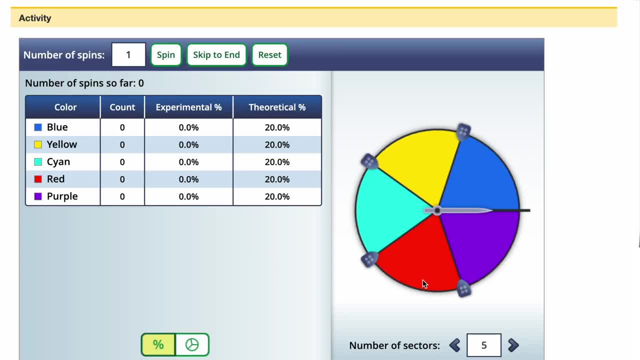 the link is in the description. You can customize your own spinner. You can decide how many sectors or sections the spinner has. You can choose the number of spins. In this case, I did 50. And maybe the best feature is that you don't have to sit there and wait until all 50 happen. 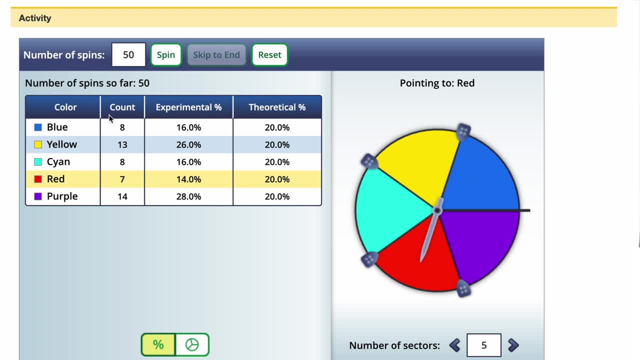 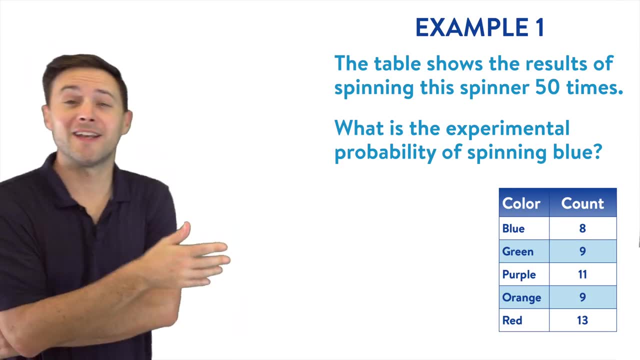 You can click, skip to the end and then it'll just show your results. So if you want to do this on your own, go to the website and give it a try. All right, so now for the question. The event is spinning a balloon. What is the experimental probability of spinning a balloon? What is the 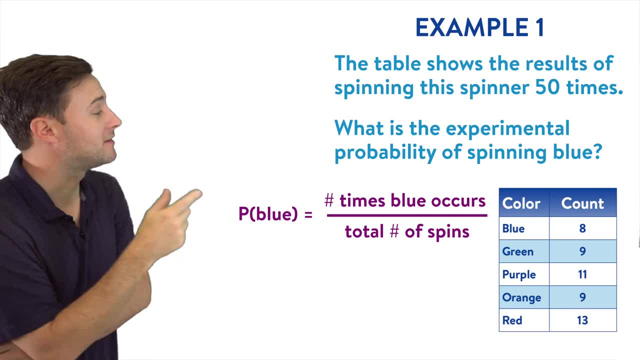 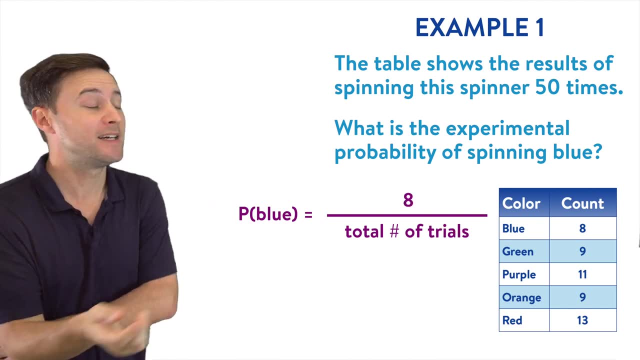 experimental probability of spinning a balloon. Well, the answer is blue. So the probability of blue- we'll put that in parentheses- is going to be equal to the number of times it landed on blue, which, if we look at the table, was eight divided by the total number of trials. Well, how many times? 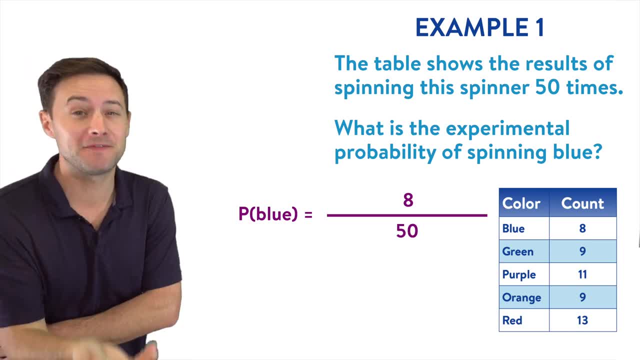 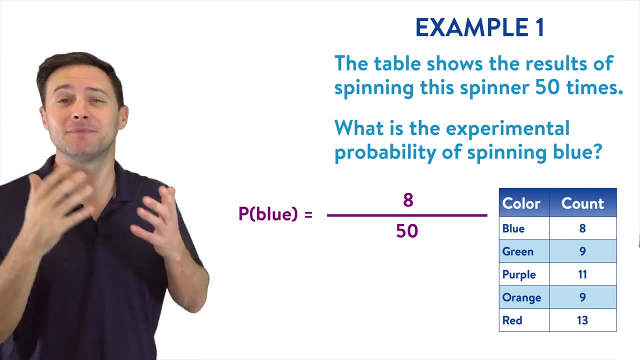 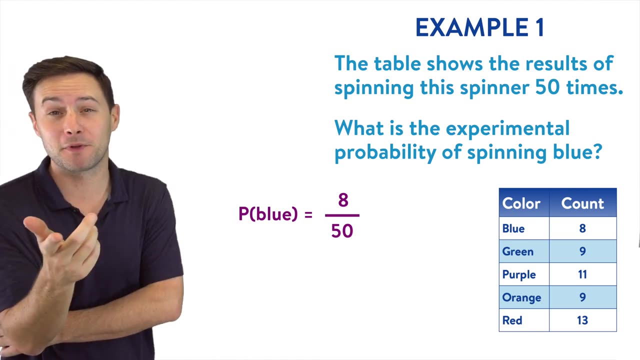 did we spin the spinner? If you remember, we spun it 50 times. You could even double check by finding the sum of all of those counts And if you add them up, the answer is 50. So the probability of blue is over 50. But we can simplify that: Divide the numerator and denominator by 2 and that gives us. 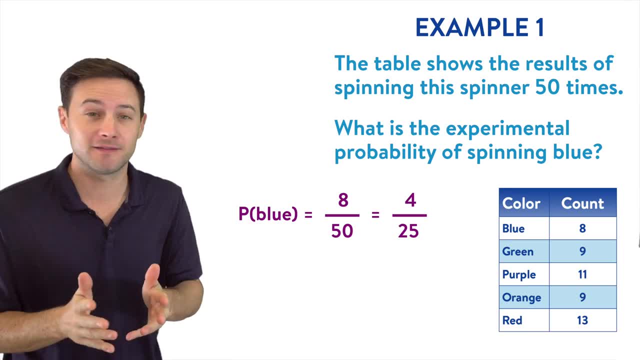 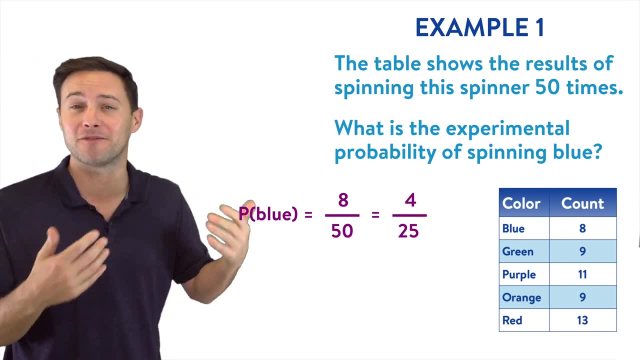 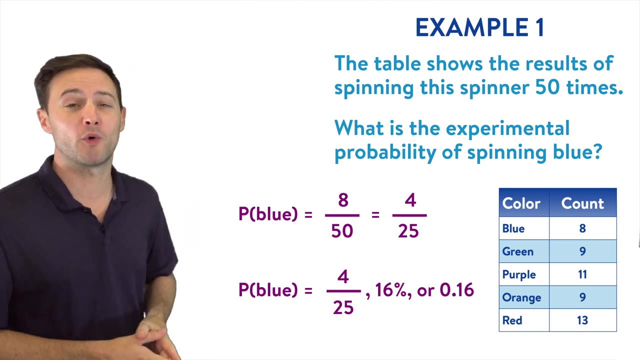 4 over 25.. That would be the fraction answer. We could change that into a percent- right Pretty easy times. numerator denominator by 4 to get it over 100, which would be 16 percent. or even as a decimal we could write it as 0.16.. Which means, out of all 50 of those spins, 16 of the time it landed on blue. 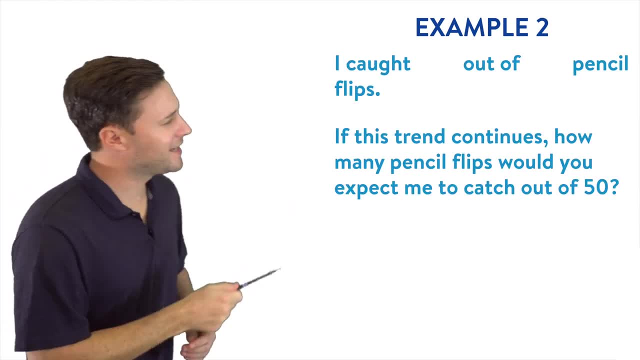 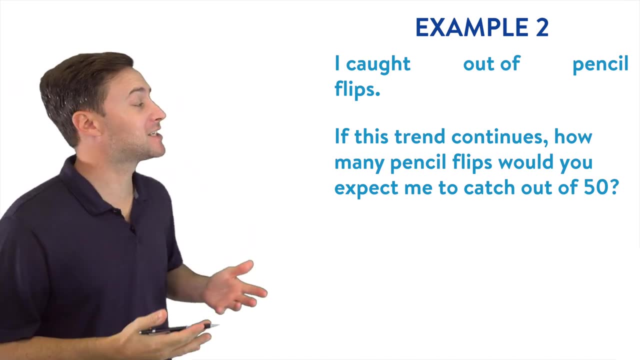 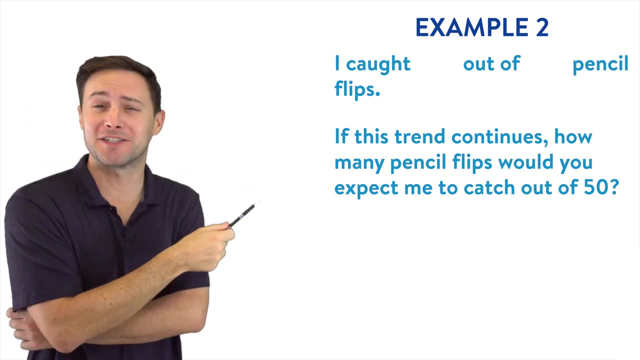 Let's try another example, Example 2.. I caught blank out of blank pencil flips. If this trend continues, how many pencil flips should i expect to catch out of 50.. Hmm, Well, that's a very good question. Notice, this question is not really finished. It says: 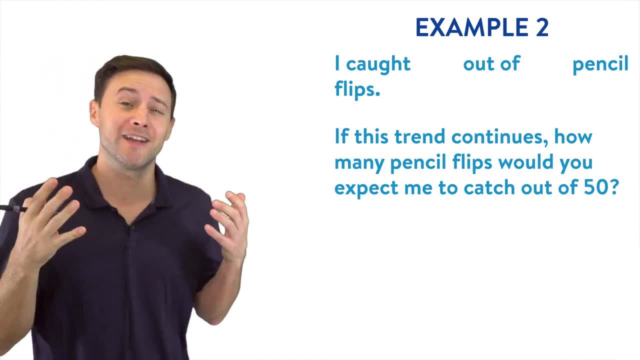 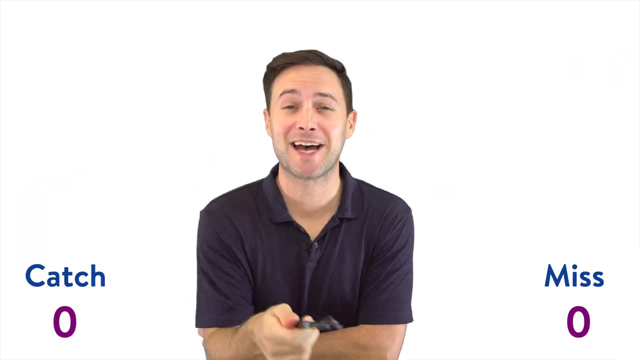 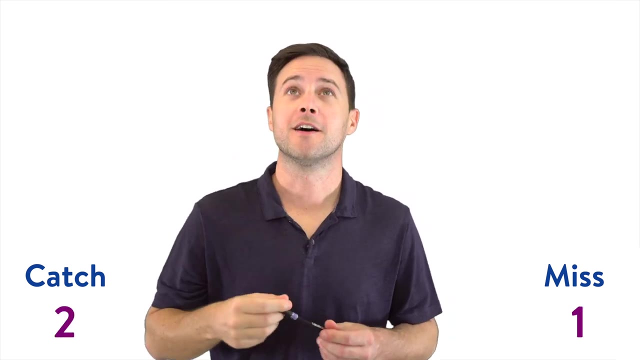 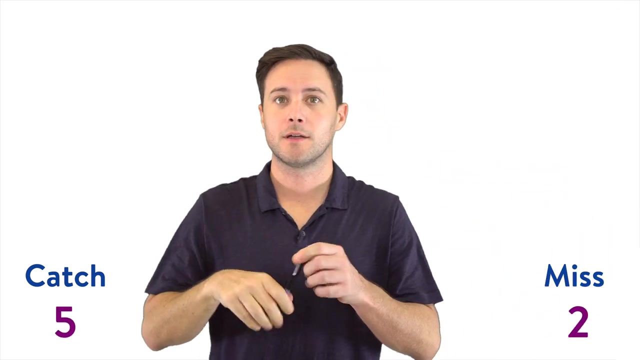 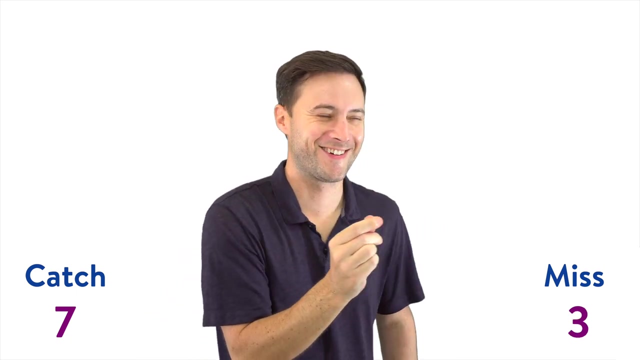 blank and blank pencil flips. so i guess to find an experimental probability, first thing I need to do is an experiment. Alright, let's collect some data. So I'm going to flip it times, see how many I catch out of ten. All right, not my best performance, maybe I'm a little bit rusty, but at least we've. 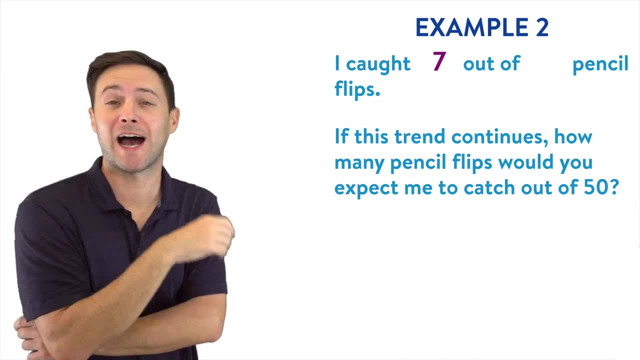 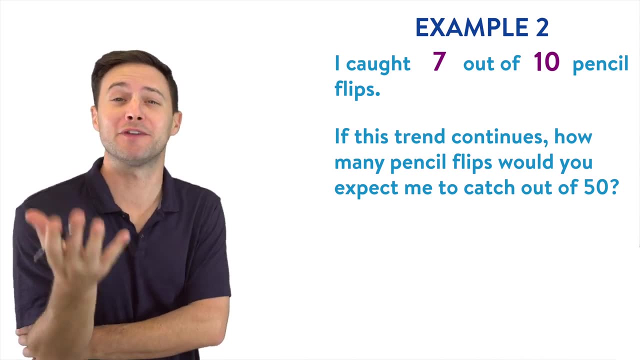 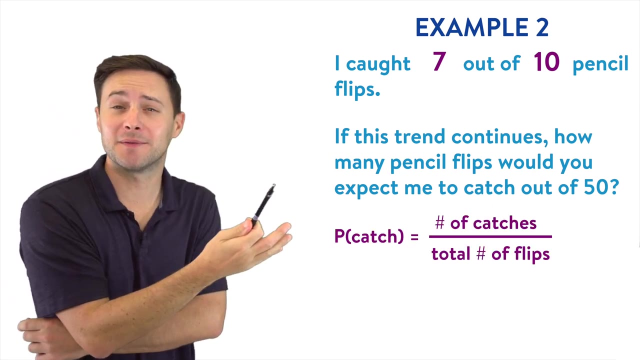 got some results. So I caught seven out of the ten pencil flips. Now we can use those results to find my experimental probability for catching a pencil flip. So probability of a catch, well, that's equal to how many times did I catch it? Seven out of. how many times did we do the experiment? How many times did I? 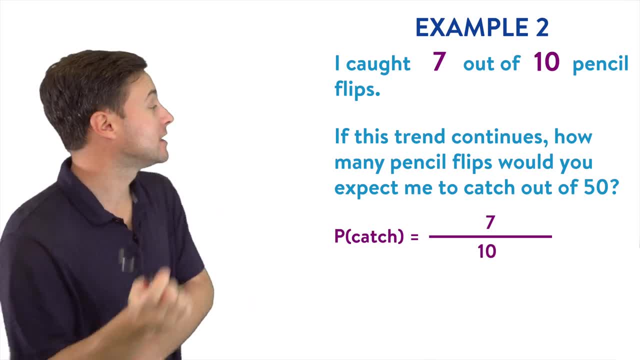 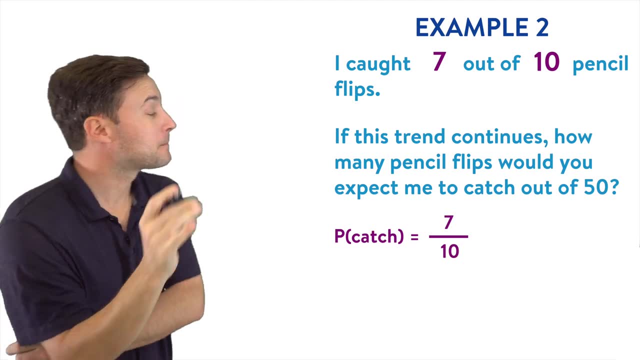 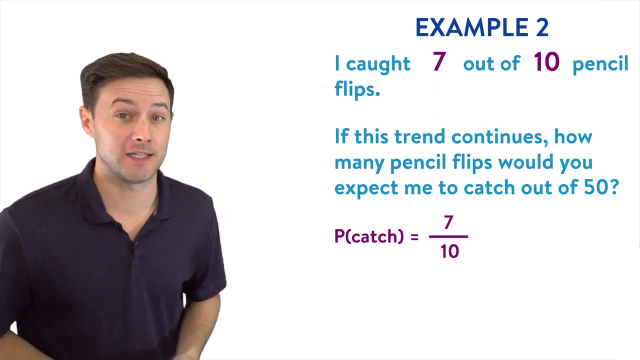 actually flip it total. Well, I did it ten times, So experimental probability of catching a pencil flip is seven out of ten. Now we need to use that to help me predict how many catches I would get out of 50.. I don't want to sit here and do 50. 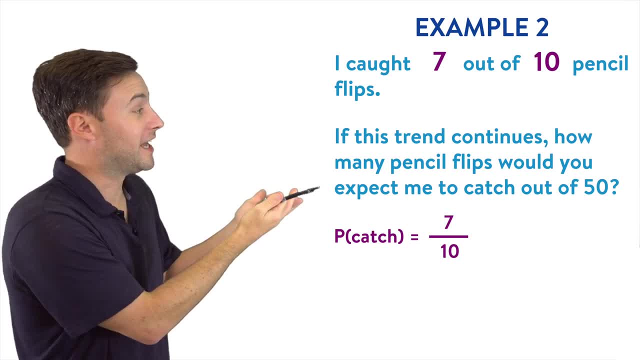 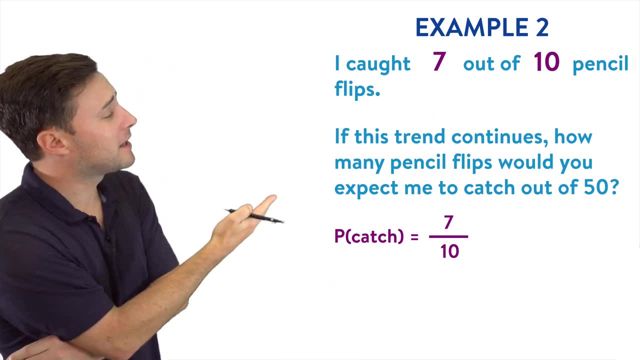 pencil flips and count all of them. I want to use the information from doing the ten to make it hopefully a good prediction. So a couple different ways we could do this. If I think about it, that experimental probability means I caught seven out of ten. 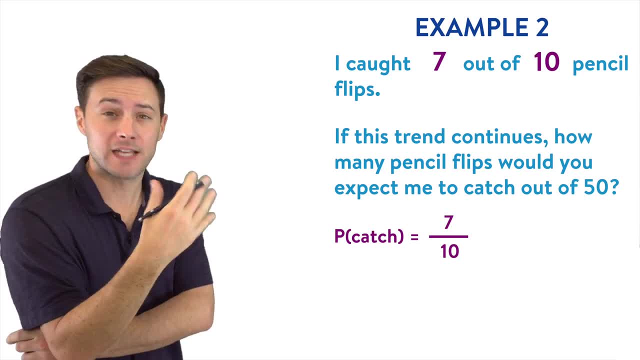 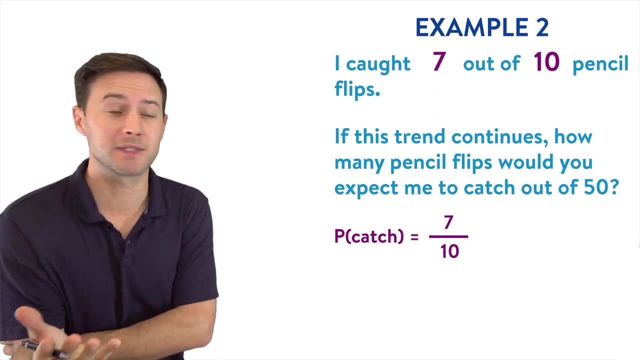 So I caught seven tenths of the flips, Right, Seven tenths or 70% or 0.7.. I caught 70% of them, or seven tenths of the flips. So if I'm doing 50 flips, I can figure. 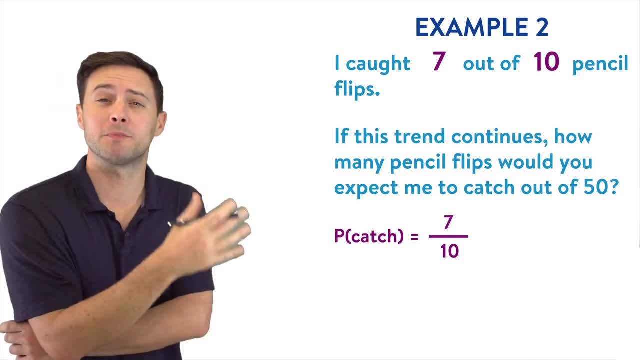 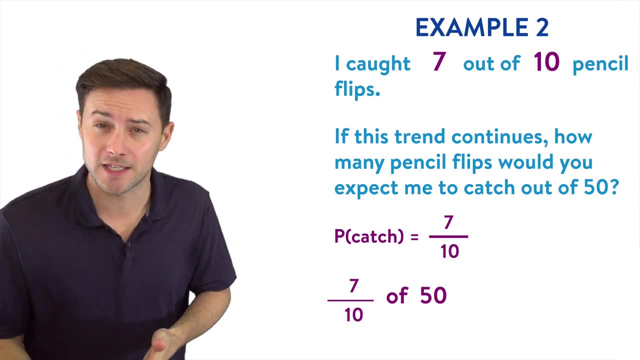 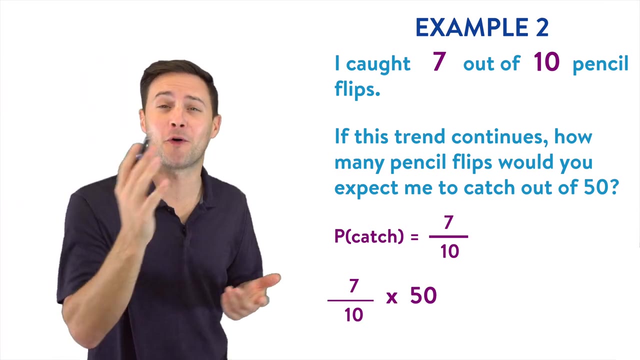 out how many I should expect to catch by just using multiplication. If you think of it this way, seven tenths of the flips, Well, seven tenths of 50. in this case, that just means seven tenths times 50. So if I do that again, before I multiply, always, always, always, try to simplify. 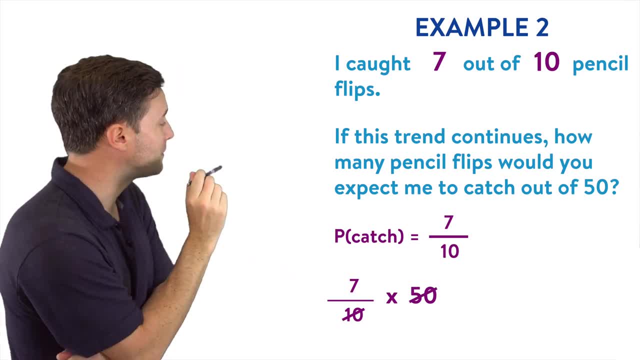 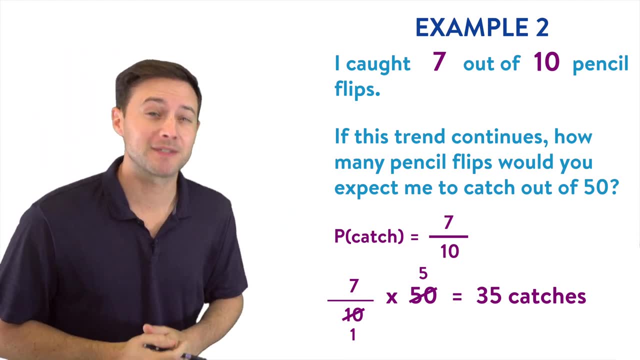 first, so I can simplify, the 10 and the 50. that becomes 1, that becomes 5.. Seven times 5 is 35. So out of 50 flips I would expect to catch 35 of them. Now here's a few to try on your own. 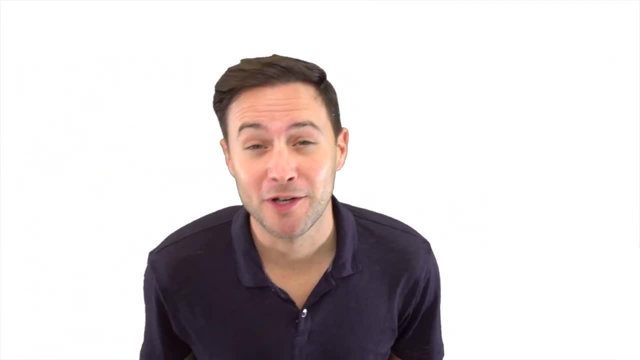 Alright, so that was experimental probability. Stay tuned for the next video to learn all about theoretical probability. 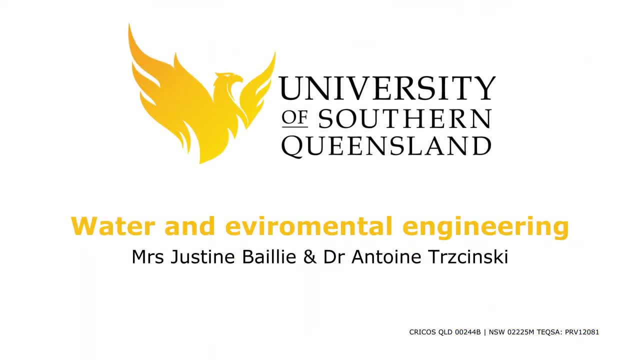 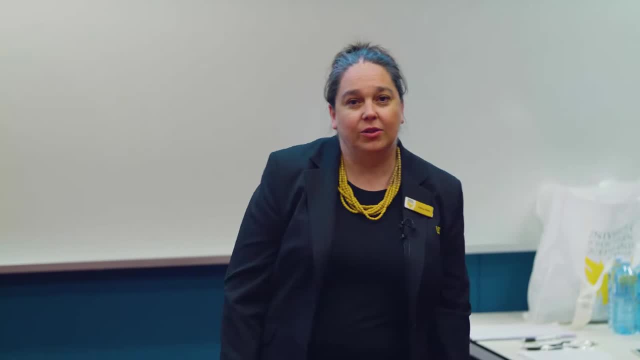 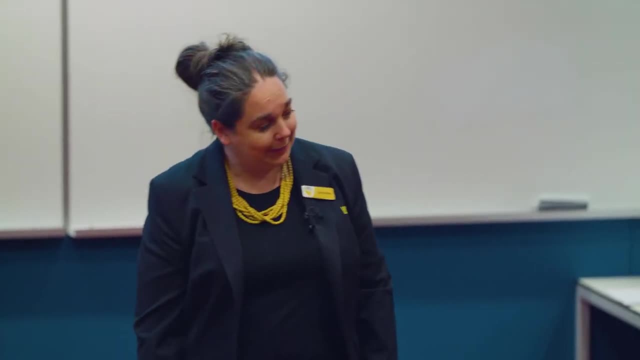 My name's Justine Bailey. As Robin mentioned, I'm with our School of Civil Engineering and Surveying. My background is actually as a civil engineer and I graduated from USQ a couple of decades ago. now I've only been full time with USQ for a couple of years. 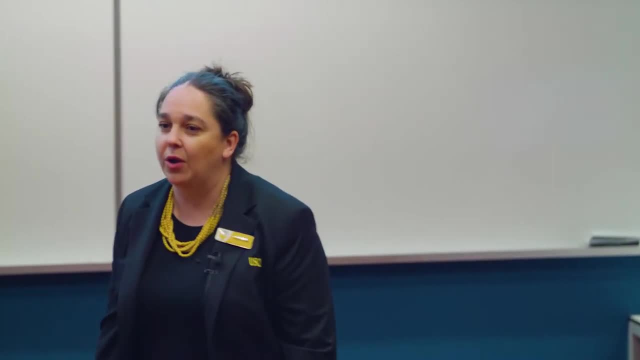 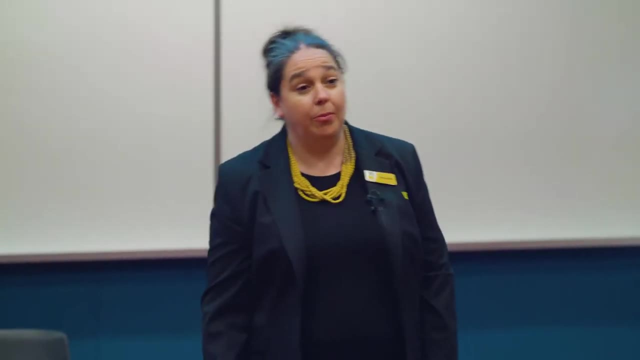 Before that, my background's actually in industry, So I was involved in working for the public sector, managing our water resources and being involved in some catchment planning, operating some of our dams in Queensland and also providing some consulting services to irrigators. So 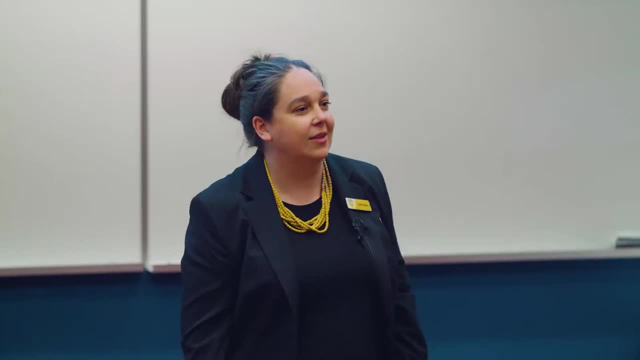 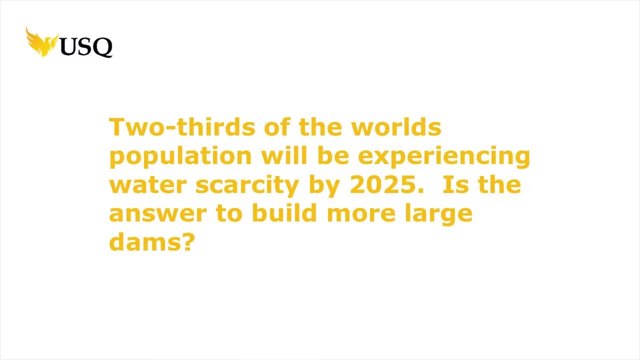 I've got a fairly broad experience in the water industry, and that's one of the things that I bring to USQ. One of the questions I get asked a lot as a water engineer, then is: should we be building more dams? There's no question that we have some challenges on. 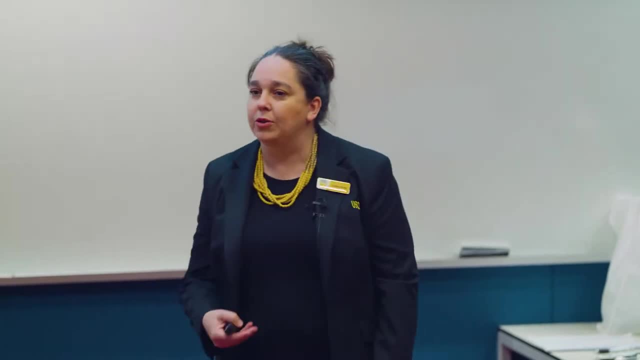 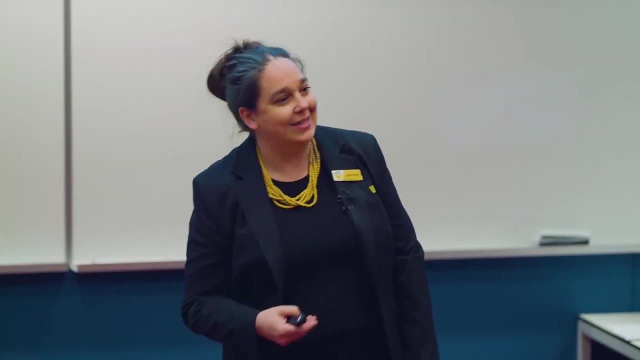 our planet in terms of water supply. A very large proportion of the population is in a situation of water scarcity, and it's a problem that's increasing. So the easy question is: should we build more dams? It's an easy question, but there's no easy answer. 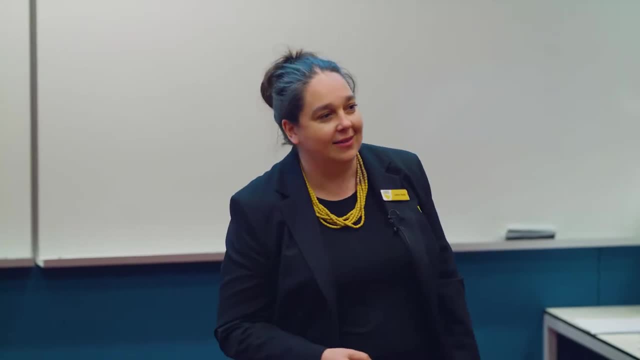 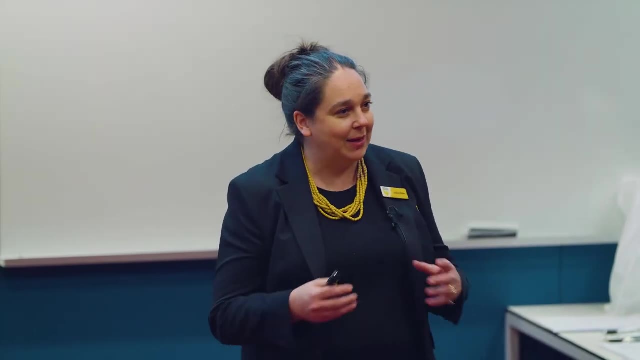 to it because it's really a complex problem and it's a complex answer that really comes into play. We're going to take that complexity and try and bring it down into maybe what some of the issues are in about the space of about five minutes. So today I'm not going. 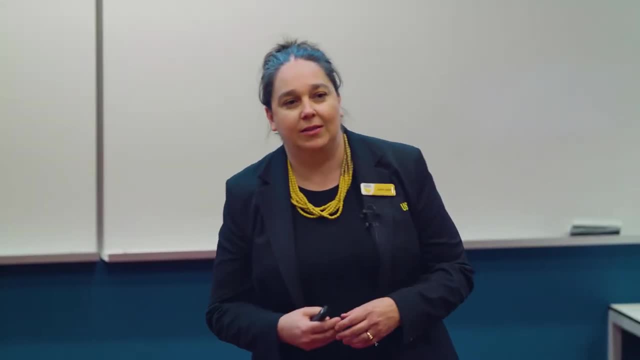 to give you the answer, but I'm going to give you a lot to think about and I'm going to give you a bit to think about in terms of if this is something you'd like to be a part of, maybe you could be a part of that. So I'm going to give you a bit to think about. in terms of if this is something you'd like to be a part of, maybe you could be a part of that. So I'm going to give you a bit to think about in terms of if this is something you'd like to be a part of, maybe you could be a part of that. So I'm going to give you